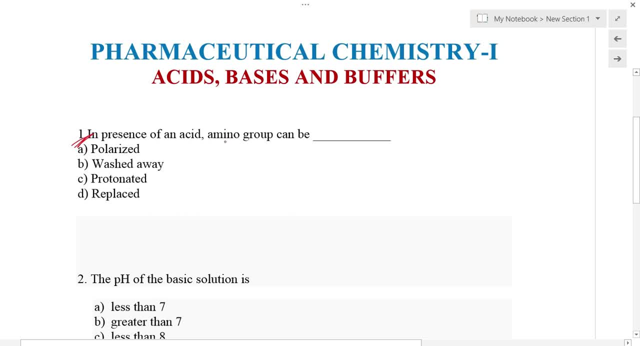 acid amino group can be: option a- polarized. option B- washed away. option C- protonated. option D replaced. the correct answer for this question is: in the presence of an acid amino group, can be option C protonated. in the presence of an acid amino group can be protonated because we 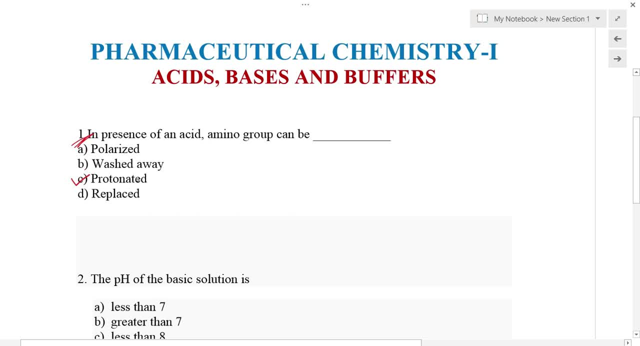 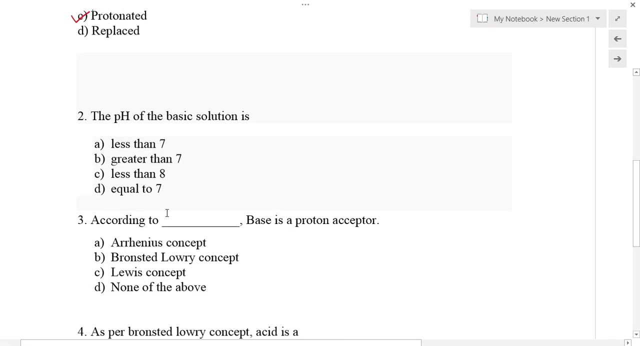 know that acid releases the proton. okay, in the presence of acid. so the amino group can be protonated. protonated because of the presence of proton, as it releases the proton. okay, now we are moving to the next question, question number two: the ph of the basic. solution is: what is the ph of basic? 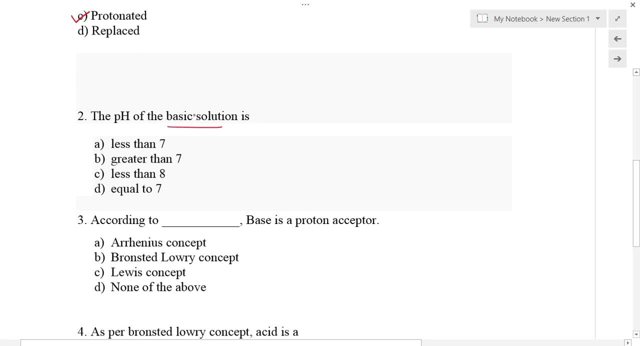 solution: simple question: option a- less than 7. option b- greater than 7. option c- less than h. option d- equal to 7. okay, the ph of basic solution. we know that basic solution has ph value greater than 7. the correct answer is option b- greater than 7. ph of the basic solution. 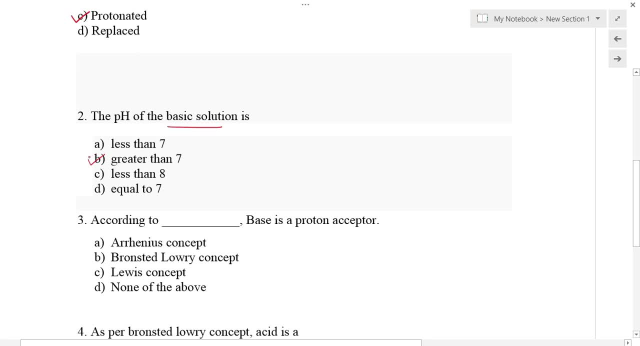 is greater than 7. what about the acidic solution? acidic solution has the ph below 7, that is, less than 7. okay, for neutral solution, it will be equal to 7. from 0 to 7 it is acidic. from 7 to 14 it is basic. okay. 7, it is neutral. okay. now we are moving to the next. 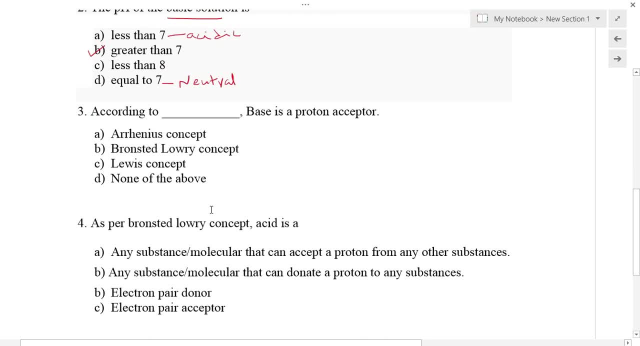 question. question number three: according to dash base is a proton acceptor? according to which concept or which theory base is a proton acceptor? option a: adenius concept. option b. bronsted lorry concept. option c- lewis concept. option d- none of the above. this is a. 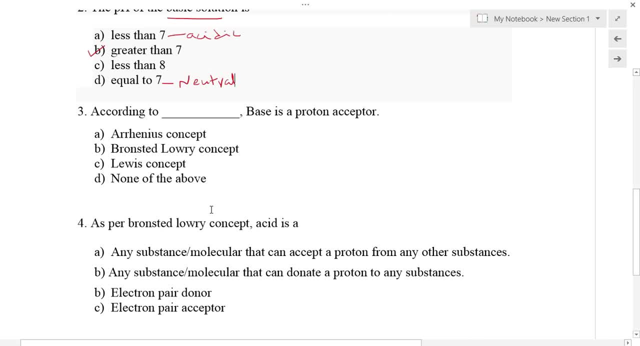 an important question and also simple question. you have to study all these concept. what is adenius concept, bronzed lorry concept, then lewis concept? this three are main theories regarding this. acids and bases. okay, we will see the answer after that. we will discuss each. according to dash, base is a proton. 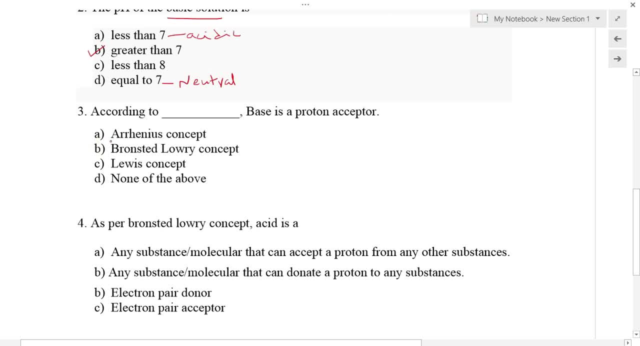 acceptor. the correct answer is option b- bronsted lorry concept. according to the bronsted lorry concept, base is a proton acceptor, acid is a proton donor. According to Bronsted-Lowry concept, acid is a proton donor and base is a proton acceptor. Now we will see what are the theories. 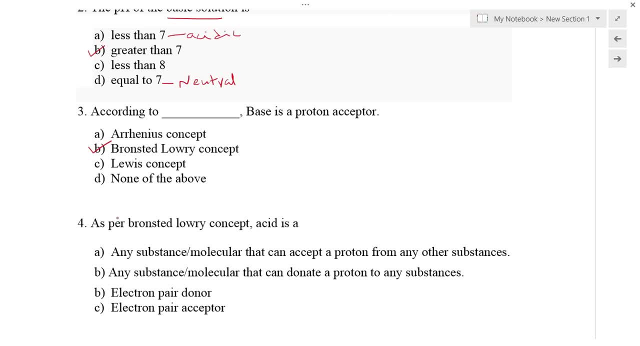 regarding acids and bases. First one is traditional theory. okay, traditional concept, then Arrhenius theory, then Bronsted-Lowry theory, then Lewis theory or Lewis concept. okay, I mean there are mainly three types, but one another one is that is traditional theory. okay, So total four theories. one is traditional. 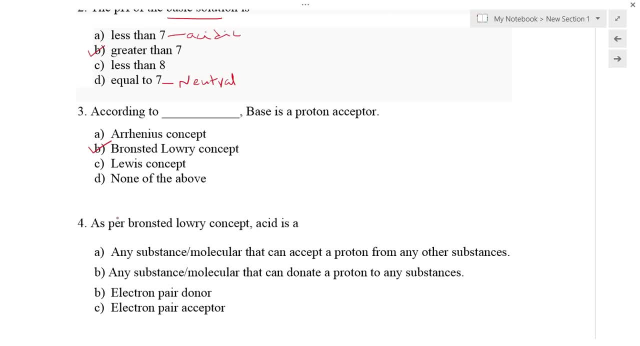 theory, then Arrhenius theory, then Bronsted-Lowry theory, then Lewis theory. total four: okay. So what is traditional theory or traditional concept? According to the traditional concept, acid will convert blue litmus paper to red. okay. 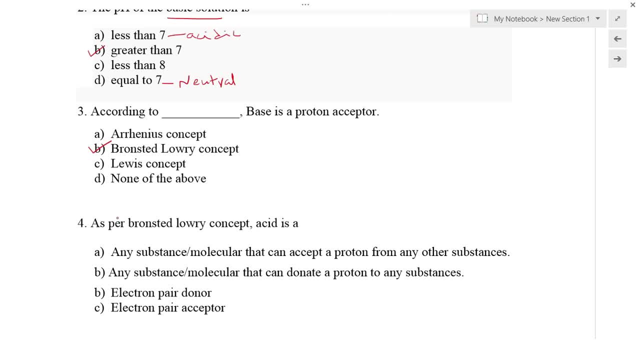 acid will convert blue litmus paper to red. okay, then the acid pH will be less than seven. then it has got sour taste. okay, these are the main important points regarding the traditional theory. okay, the next one is base. according to the traditional theory, base base will convert. 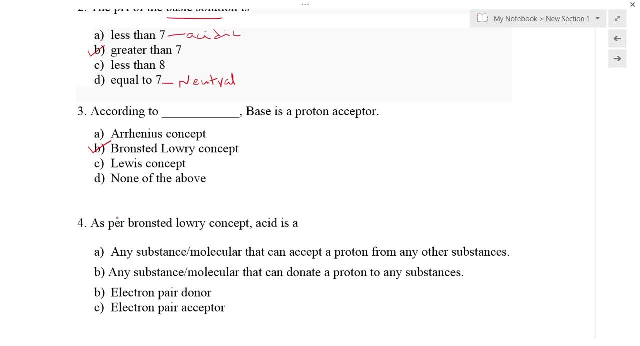 red litmus paper to blue. okay, it will convert red litmus paper to blue. and also, it has got bitter taste. it has got bitter taste and the ph will be greater than seven. okay, that is the traditional concept according to the arenas theory. that is the second theory, arenas theory. 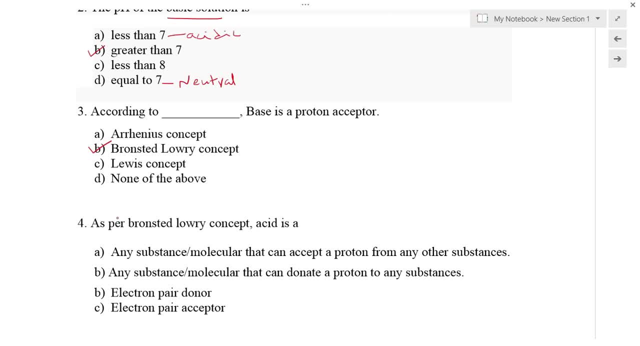 or arenas. concept acid is those who generates the hydrogen ion- okay, those who generate hydrogen ion or h plus ion- okay, you had to note that here. acid which will generates- okay, generates, not donates- okay, acids are those which generates hydrogen ion- okay. second one is base, that is, base which generate. 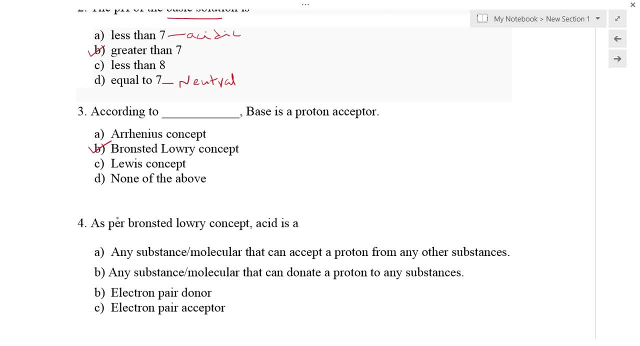 hydroxyl ion. this is the arenas concept. according to the arenas concept base, will generate hydroxyl ion. acids will generate hydrogen ion. the next one is bronsted lori concept. that was the question. according to the bronzed lori concept, acid is those who donates the h plus or who donates the proton. okay, acid is who donates the proton basis. 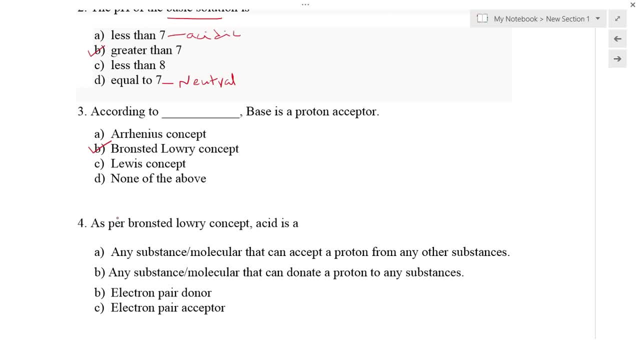 who accept the proton. So acid is a proton donor and base is a proton acceptor. That is the Bronsted-Lowry concept And the last concept, that is Lewis theory or Lewis concept. According to the Lewis concept, acid is electron pair acceptor. 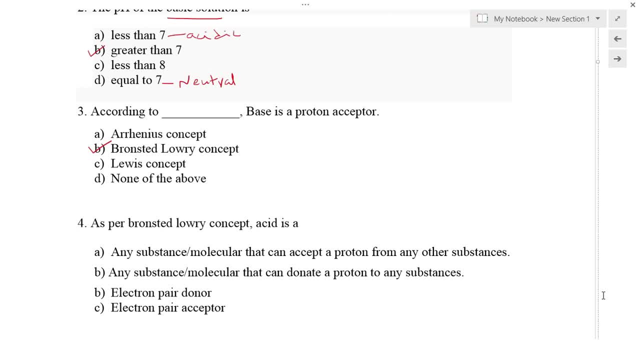 According to the Lewis concept, acid is an electron pair acceptor and base is electron pair donor. Okay, electron pair donor. These are the main concepts regarding the acids and bases. One is traditional concept, then Arrhenius concept, then Bronsted-Lowry concept, then Lewis concept. 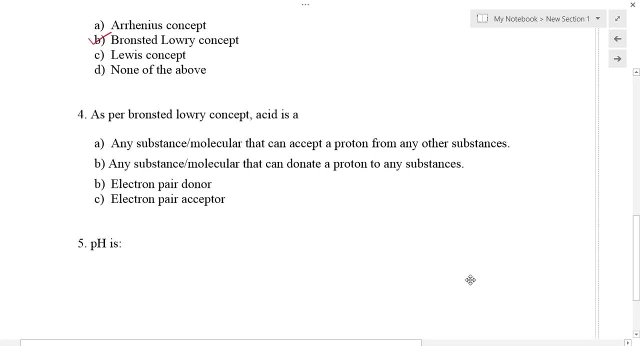 Now we are going to the next question, question number four. As per Bronsted-Lowry concept, acid is a option A: any substance or molecule that can accept a proton from any other substance. Option B: any substance or molecule that can donate a proton to any substance. 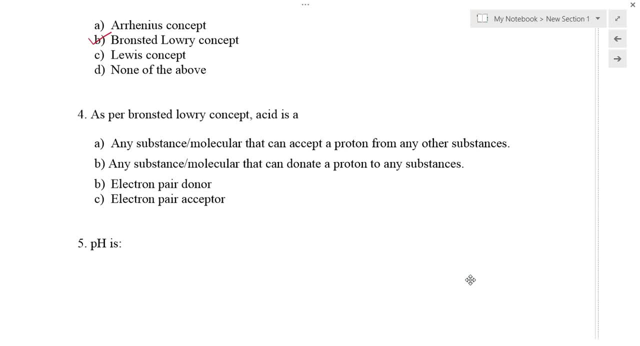 Option B- electron pair donor. Option C- electron pair acceptor- Bronsted-Lowry concept- Uh, according to the Bronsted-Lowry concept, acid is an option B. is the correct answer any substance or molecule that can donate the proton. 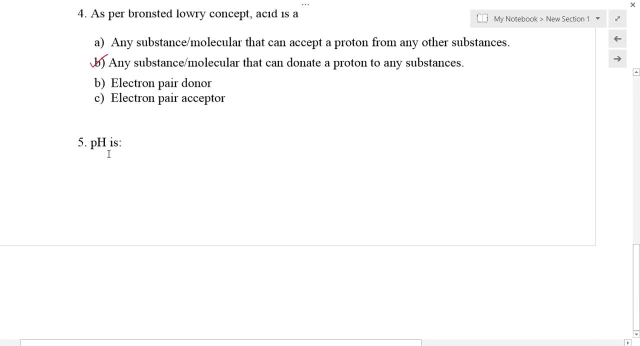 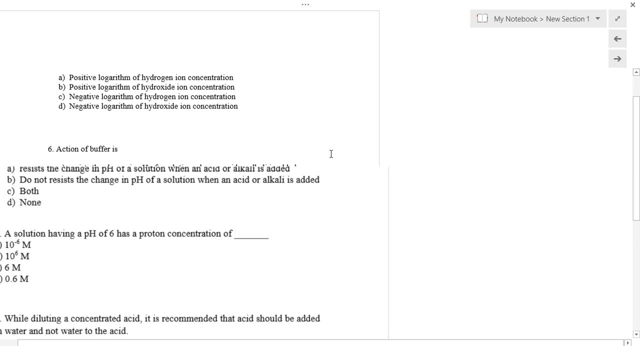 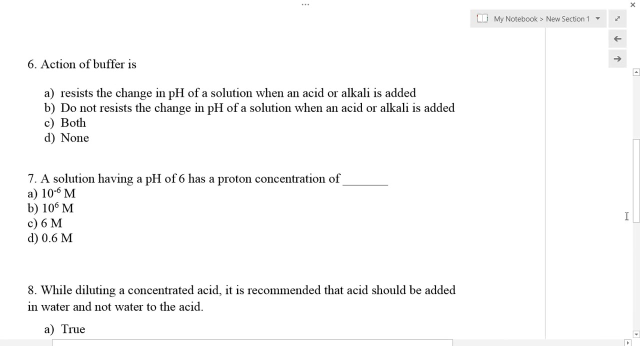 Proton donor, that is, the acid in case of Bronsted-Lowry concept. Question number five: pH is pH is option A- positive logarithm of hydrogen ion concentration. Option B: positive logarithm of hydroxide ion concentration. 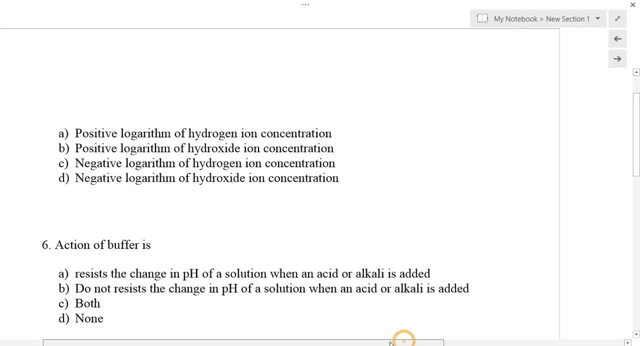 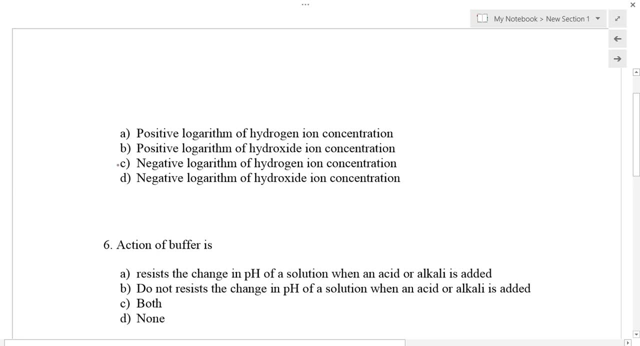 Option C: negative logarithm of hydrogen ion concentration. Option D: negative logarithm of hydroxide ion concentration, pH. we know that pH is negative log of S3O plus concentration. That is, option C is the correct answer. Negative logarithm of hydrogen ion concentration. 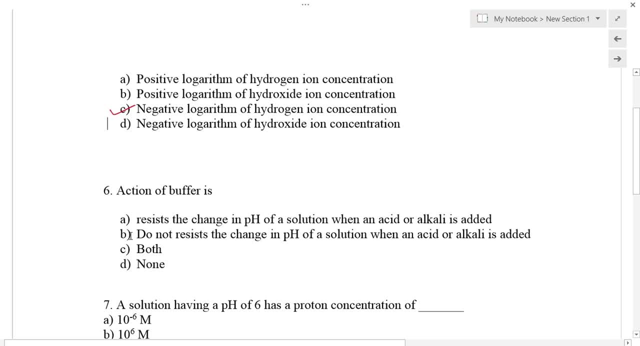 That is the pH. okay, pH. okay. pH is equal to negative log of S3O plus or negative log of H plus. okay, Now we are moving to the next question, question number six: Action of buffer is what is the action of buffer? 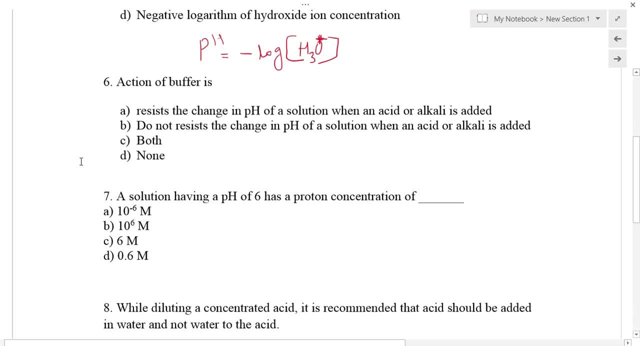 What buffer will do? Option A: resist the change in pH of a solution when an acid or alkali is added. Option B: do not resist the change in pH of a solution when an acid or alkali is added. Option C: both. 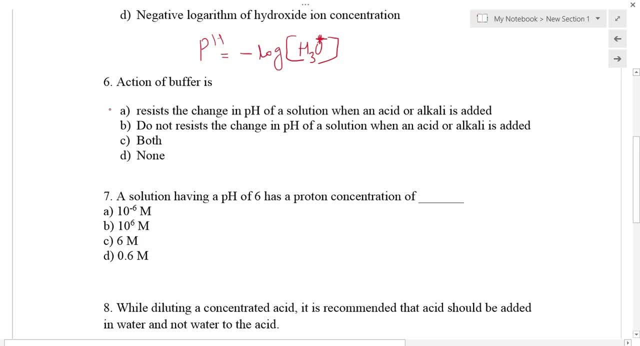 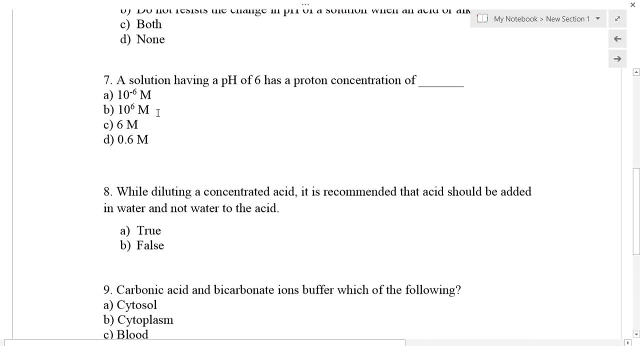 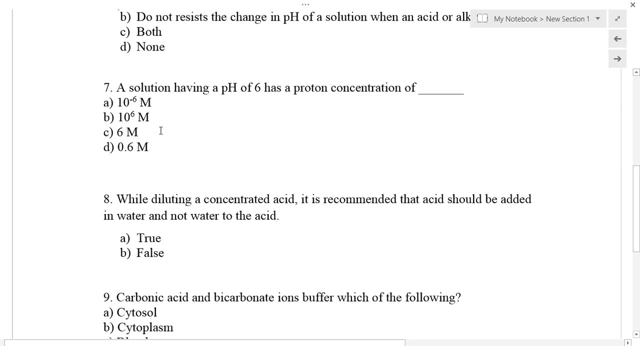 Option D: none. We know that buffer will resist the change in pH of a solution when acid or alkali is added. The correct answer is option A. Option A is the correct answer. Question number seven: A solution having a pH of 6 has a proton concentration of a solution having a pH of 6.. 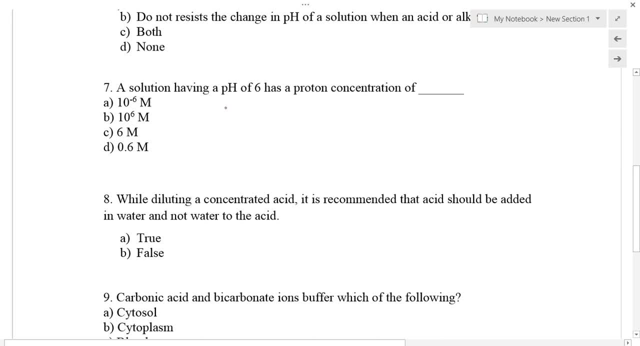 In this question, pH is given 6.. So what is the proton concentration? We know that pH is equal to negative log of H plus concentration. okay, So when we are converting, H plus concentration is equal to 10 raised to minus pH. 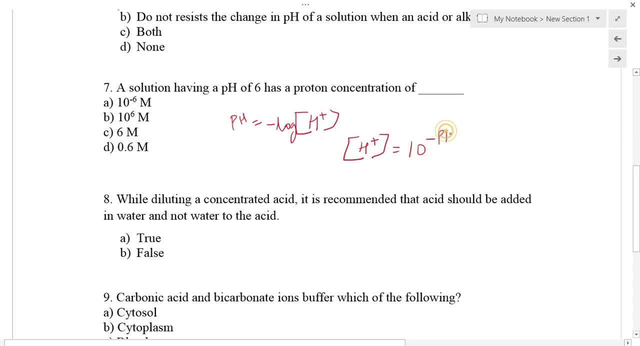 Am I correct? Okay, Then here the answer will become option A, that is 10 raised to minus 6 molar. That is here it is given. 6 is the pH. okay, 6 is given as pH. So H3O plus or H plus concentration is equal to 10 raised to minus 6, okay. 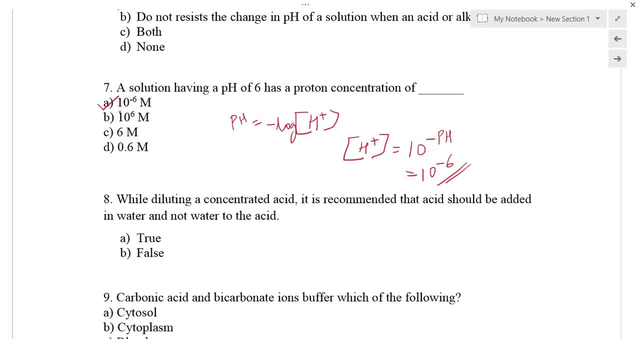 So that is the pH. pH is given 6.. So correct answer is 10 raised to minus 6 molar. We know that pH equals negative logarithm of proton concentration. Since the pH scale is logarithmic, an increasing of one pH unit corresponds to tenfold decrease in the hydrogen ion concentration or proton concentration. 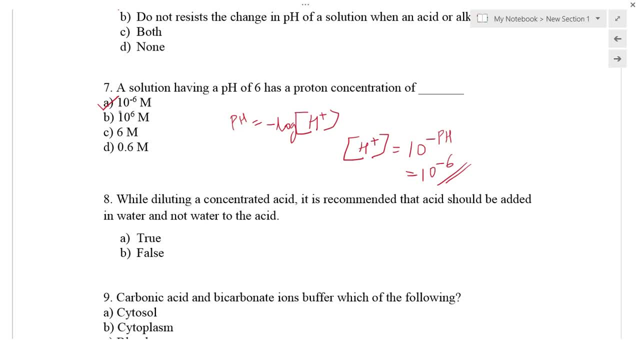 You have to note this one: We know that pH scale is logarithmic because pH is equal to negative log of H plus. So an increasing one unit of pH that will be correspond to tenfold decrease in the hydrogen ion or proton concentration. So the question maybe will come like this also: 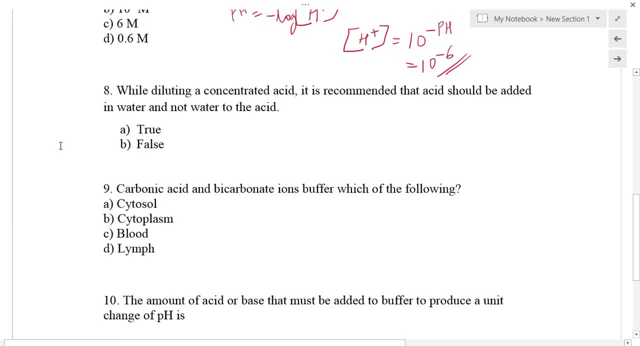 Next question, question number 8.. While diluting a concentrated acid, it is recommended that acid should be added in water and not water to the acid. okay, While diluting a concentrated acid, it is recommended that acid should be added to the water and not water to the acid. 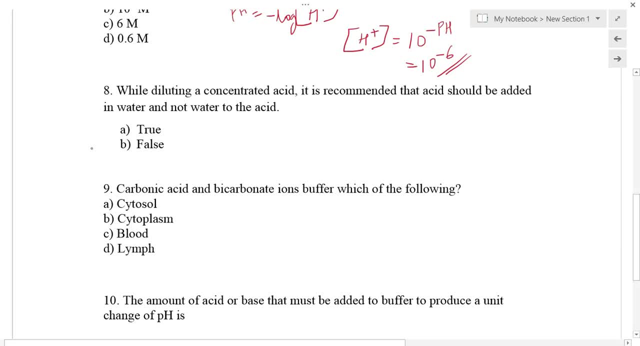 Option A: true. option B: false. Option A: true. option B: false. Okay, true or false. The correct answer is true. Option A is the correct answer. When we are diluting a concentrated acid, we should add concentrated acid to the water, not water to the acid. 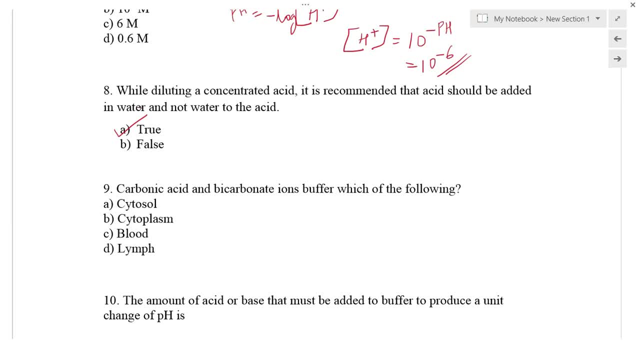 Why? Because adding water to the concentrated acid, it will make the solution to boil violently and it will splash the concentrated acid out of the container, So it will be dangerous. Okay, So don't add water to the concentrated acid. when we are diluting the acid, You should add acid to. 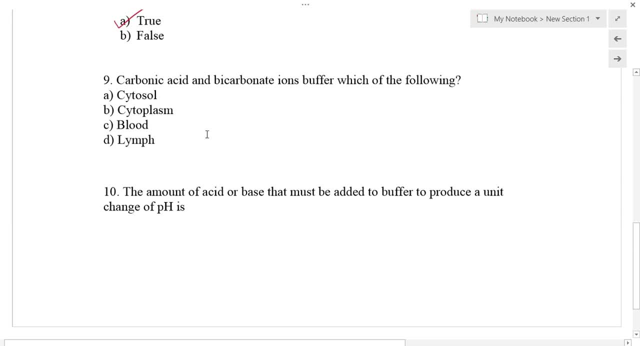 the water. Next question, Question number 9.. Carbonic acid and bicarbonate ion buffer. which of the following: Carbonic acid and bicarbonate ions will buffer which of the following: Option A- Cytosol. Option B- Cytoplasm. Option C. 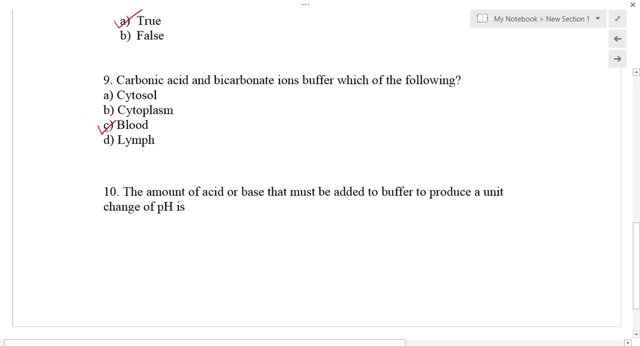 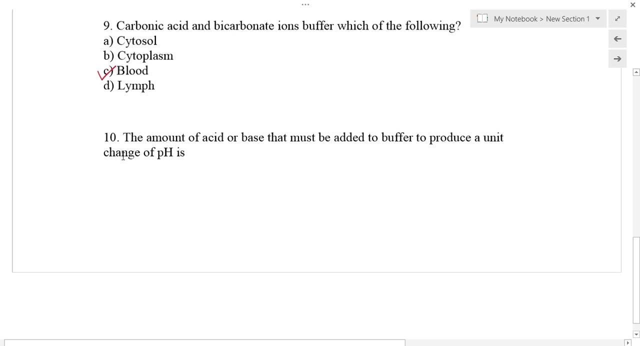 Blood. Option D: Lymph. The correct answer is option C, That is, blood. Carbonic acid and bicarbonate ion buffer the blood and hold its pH around 7.4' Okay, What is the blood pH? 7.4' Okay. And here carbonic acid is a weak. 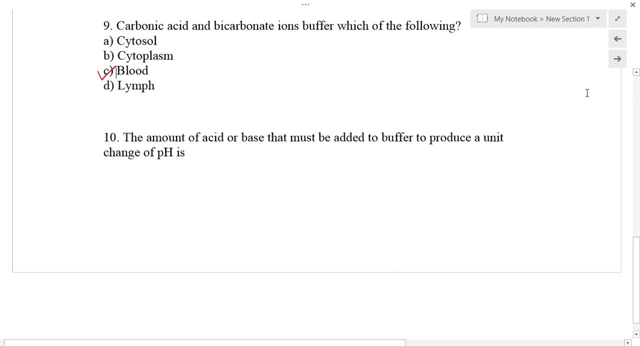 acid and bicarbonate is a base struggle in nature. Question number 10.. The amount of acid or base that must be added to the buffer to produce a unique change of pH. The amount of acid or base that must be added or not must be added to the buffer. The amount of acid or base must be added or 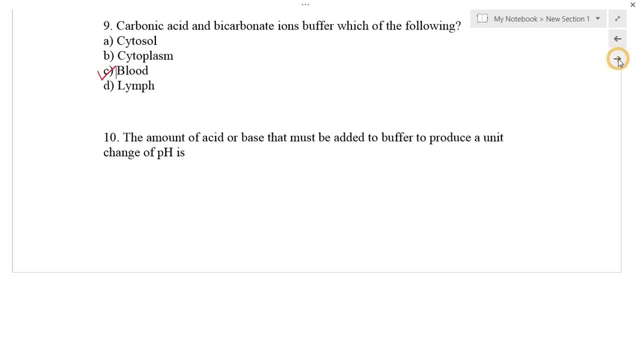 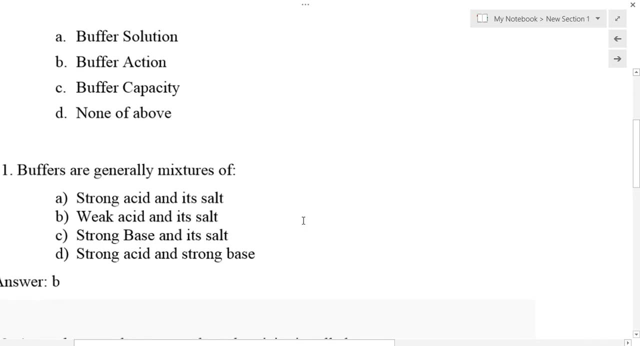 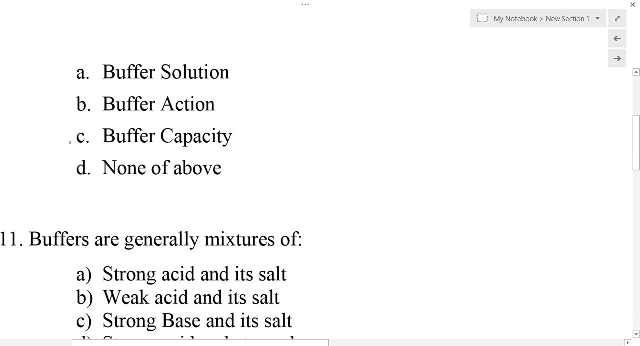 to the buffer to produce a unit change of pH. what is that term? option a: buffer solution. option B: buffer action. option C: buffer capacity. option D: none of the above correct answer is. we know that option C, that is, buffer capacity, is the correct answer. okay, thank you very much for watching this video, if you like this. 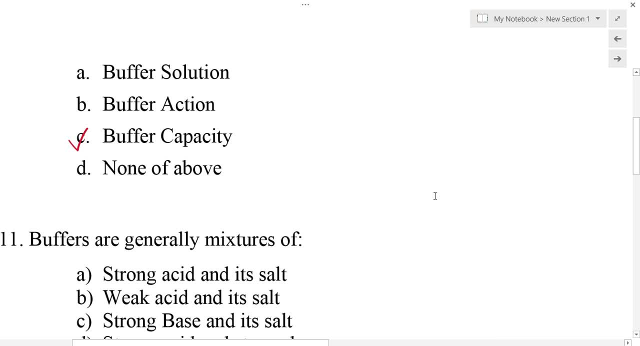 video. please make thumbs up and also subscribe the channel if you didn't subscribe until now, and also press the bell button. thank you.